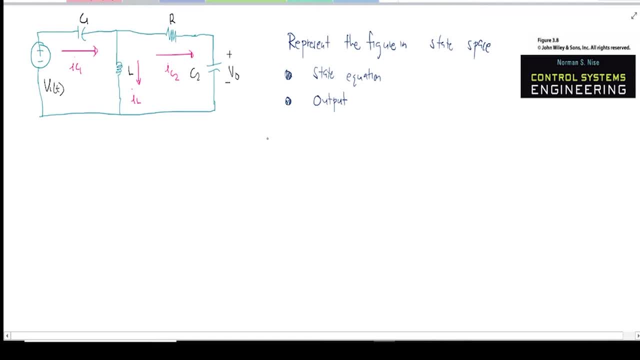 in order to fully understand what we're going to do is we're going to solve this symbolically, okay. so first things first, we should label the current, because that is important. so that's why I've already labeled this IC1, IL and IC2. okay, after this, we're going to write the equation of: 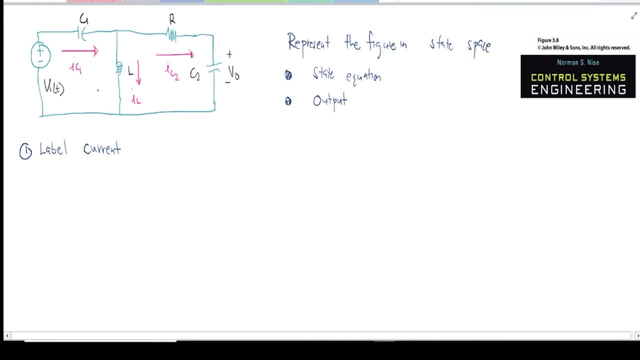 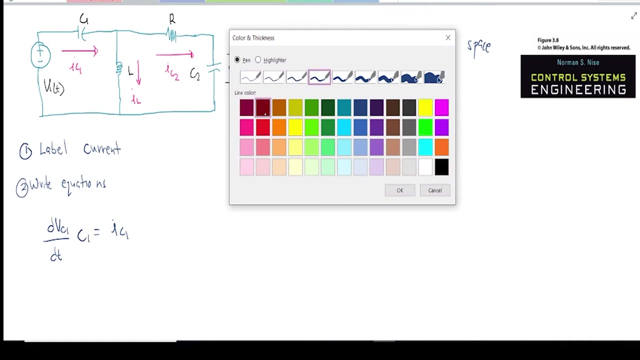 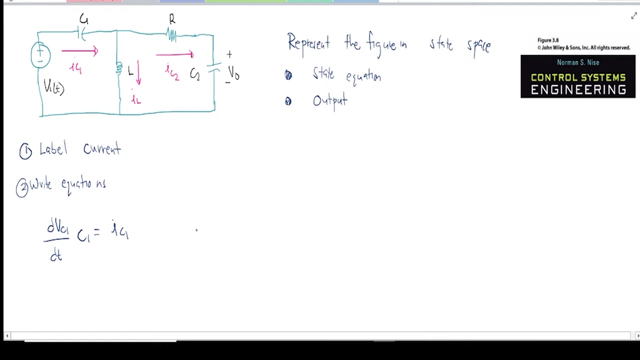 the storage components, just like capacitors, inductor and then again capacitors. so in this case the equation would be- I'm going to write the equation- or current for the capacitor one. the next equation would be for the inductor: the voltage drop in the inductor and the third one would be the current in the capacitor two. okay, so one. 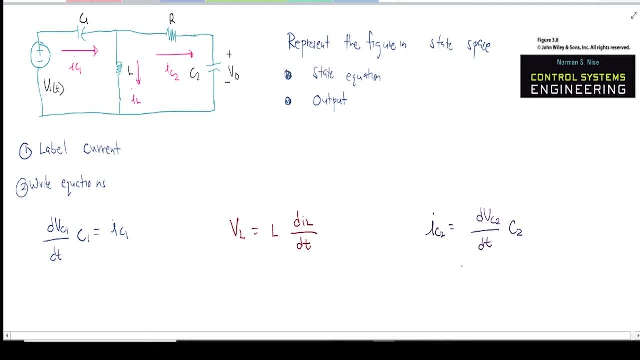 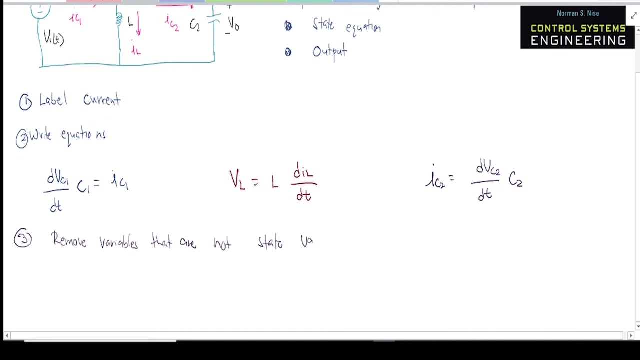 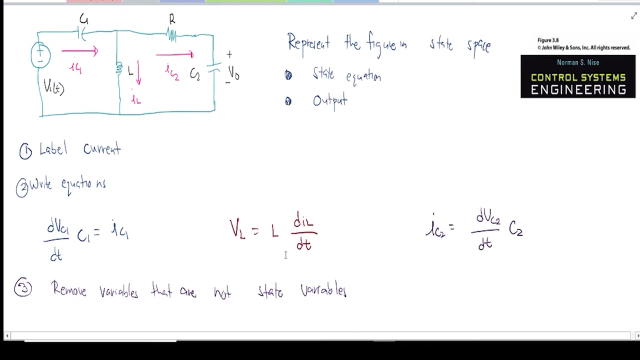 key tip when solving this kind of problem: you should be very organized and getting subscript and then organizing your stuff. okay, so the next thing to do is this one: okay, so in this problem, we're going to remove the variables that are not state variables, so an example of which would be this one, this one and then this one. 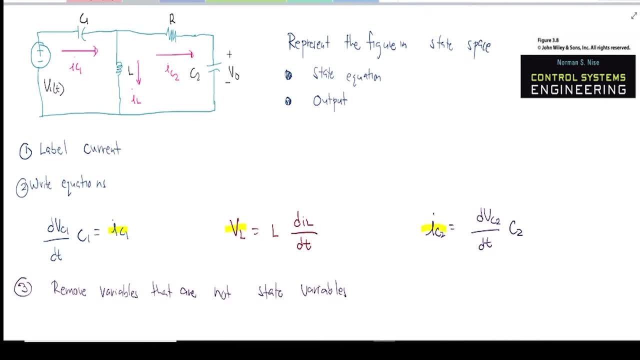 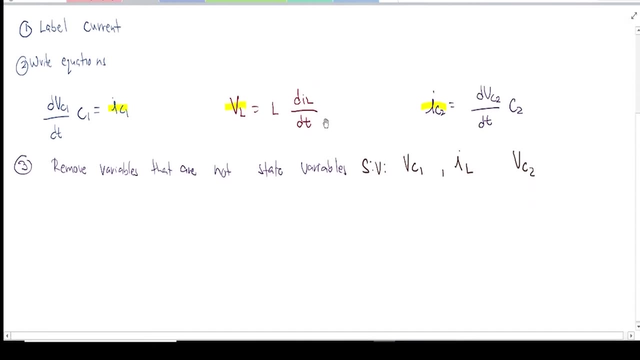 because our state variable is okay. so this are the state variable that we are concerned of so that we could okay. so these are the state variables that we are concerned of so that we could give or make some state equation okay. so this is just an easy problem. so if you 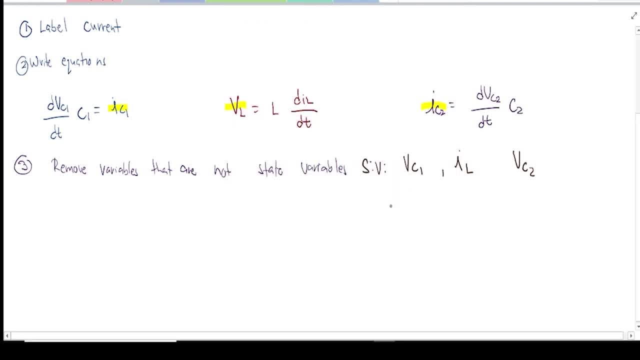 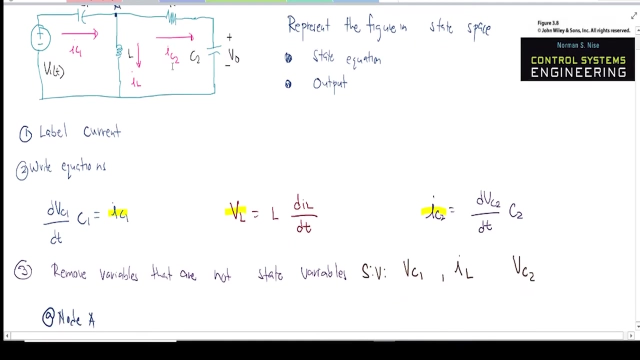 follow along. you could easily understand this concept. I assume that you have full knowledge there. the circuit, okay, so let's begin. so at node a, node e. so where is the node a? the node a would be this one, and if we're going to write the equation, the equation for the node a would be: 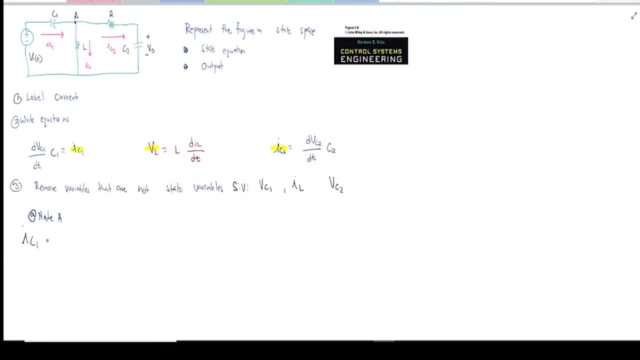 okay, so that's our um acl for the equation at node a. okay, you might be wondering why we have to find the equation in node a. it's because we're currently working on this equation. so we are working on this equation and we know that this one is not state variable, the ic1 or the current incapacitor one. 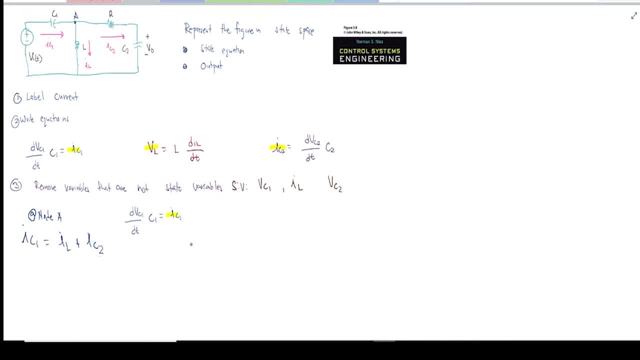 so we have to represent this ic1 in terms of state variables. so this one is a state variable. however, ic2 is not a state variable, so what we're going to do here is that think of something that we could represent the ic2. okay, let's try to analyze this loop here. 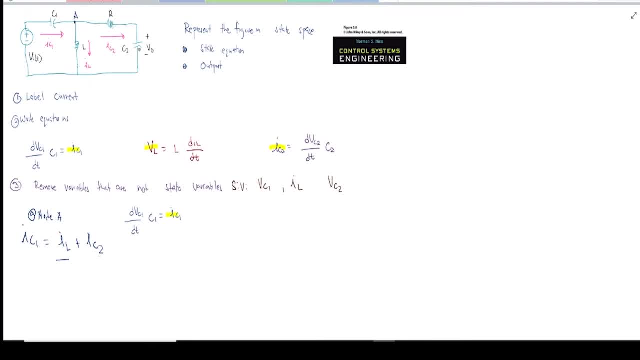 so l, r and then o, so or the output. if we try to do some kvl, what happens here is that we're going to have voltage in the voltage drop in the inductor, which is not a state variable. okay, so let's try to look the outer circuit. 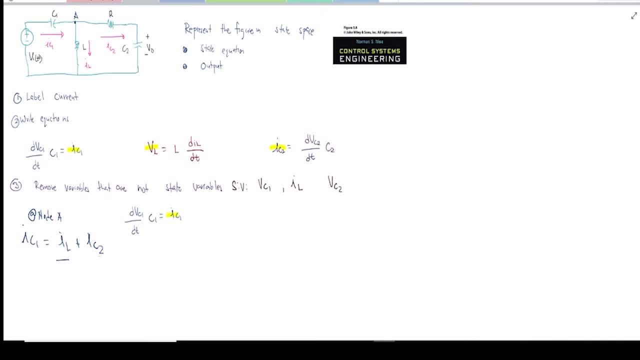 if you try to loop in this outer circuit, what will happen is that we have our input, okay, so it is part of the state equation, so we don't have to worry about this. vc1- vc1 is a state variable- okay, good. and then vr- vr is not a state variable. however, 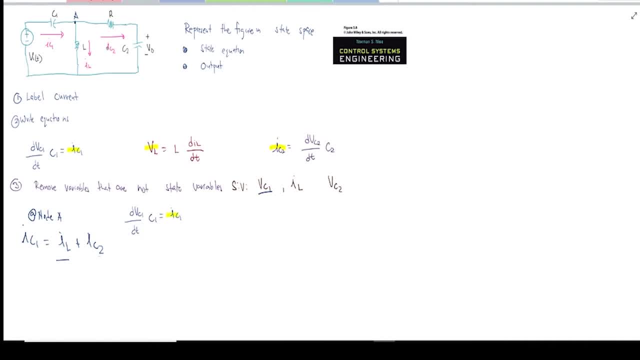 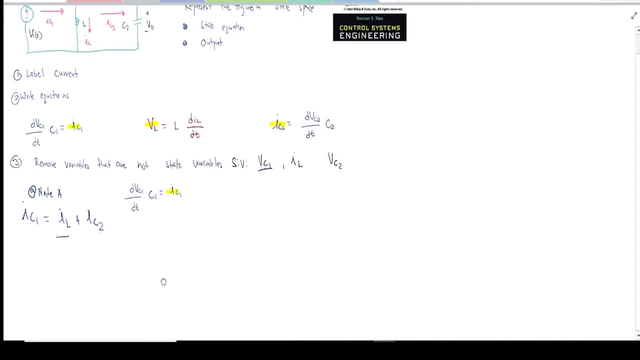 if we make the according to the solution, then we could make something out of this, because we are looking for a substitute of ic2 and then vc2 is a state variable, so we're working with um roughly 90 percent of tests in the state variable. okay, so let's put this in action. in action, if we make the. 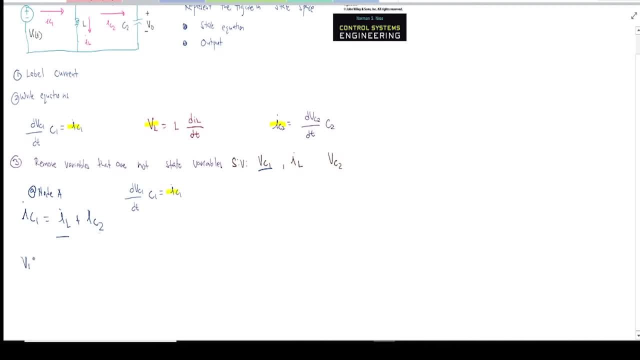 loop, the answer would be this one. okay, so that's why i chosen this loop, because, as you can see, this one is a state variable and this one is a state variable and we're concerned with the current in capacitor 2, so we have this one. we could just isolate this and then transfer all of 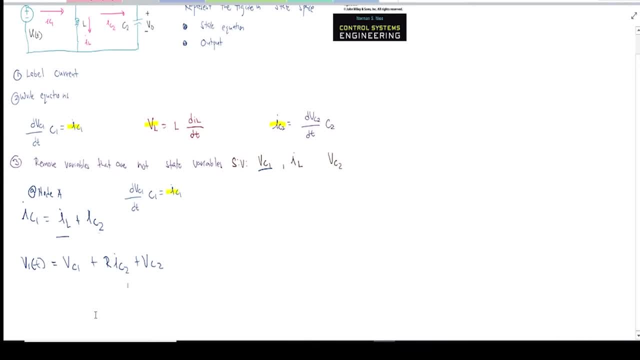 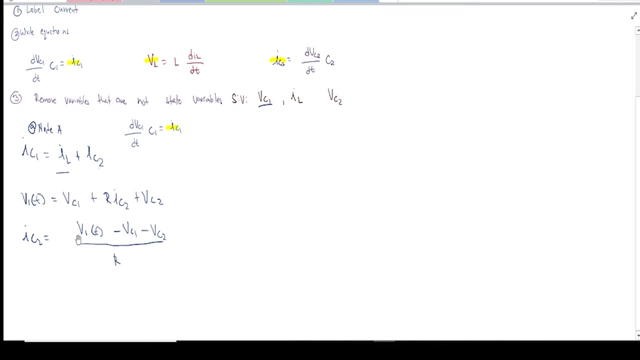 this state variable into other side. so what happens here? that it would become okay. so we already have an equation for the capacitor 2, which is, in turn, we're going to go back into this equation. so therefore, if we put this and then this into this one, 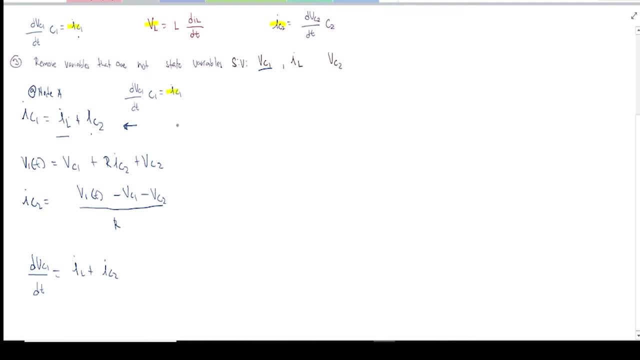 okay, that's one, and then this is not a state variable, so we're going to replace it with this one which is a state variable. okay, we're going to add the c1. it should be right here. okay, so what happens here would be cv c1. 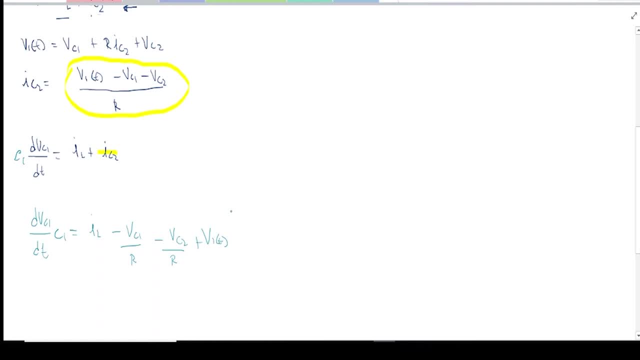 okay, and then if we multiply all of this by c1, we will have only this one on the other side. okay, so, because that's our goal for this one also, we're going to arrange it starting from our equation, one which has a state variable of vc1. 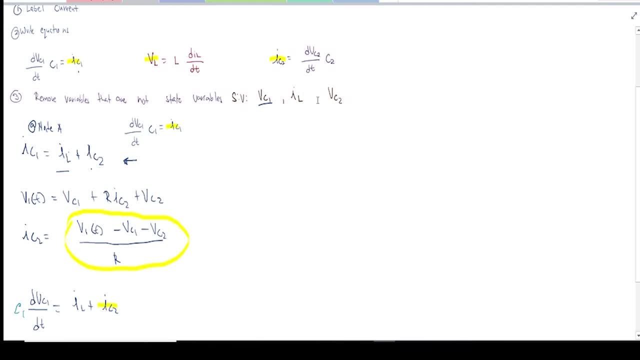 followed by iel and then followed by vc2, so that it will become a state variable of vc1, followed by the in, so that it will become a c1, so that it will become a state variable of vc1, followed by iel, then followed by vc2. 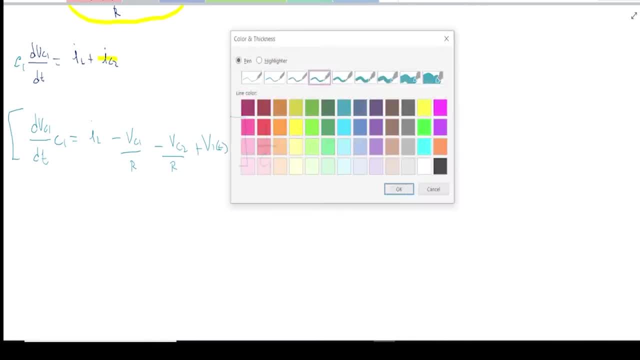 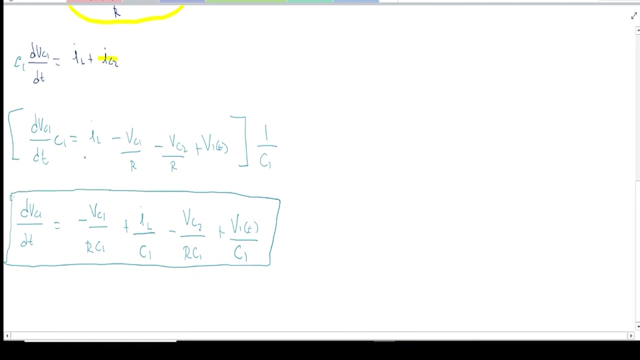 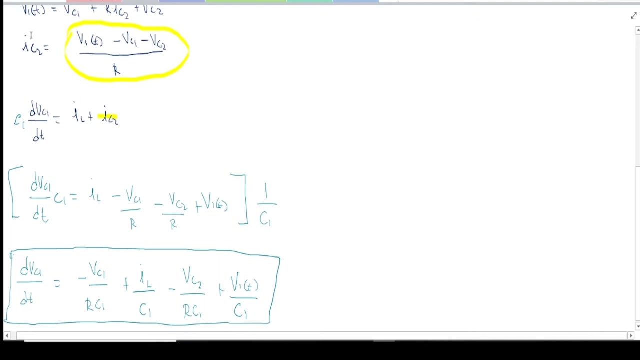 year for us in the end of the equation. okay, so, as you can see, we have now this equation and we're finished with the first equation. last two more the last two equation is just pretty easy because we're almost done with the hard stuff. the hard stuff so far is finding this current here. okay, also be aware of your. 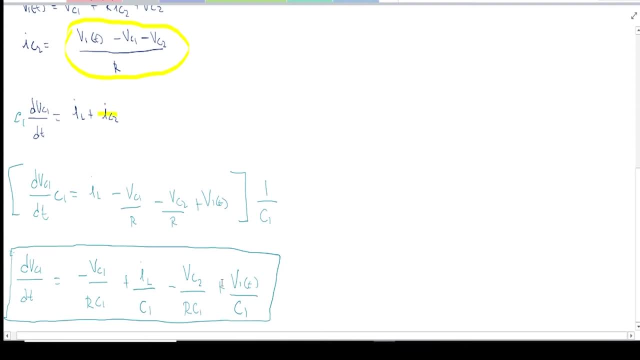 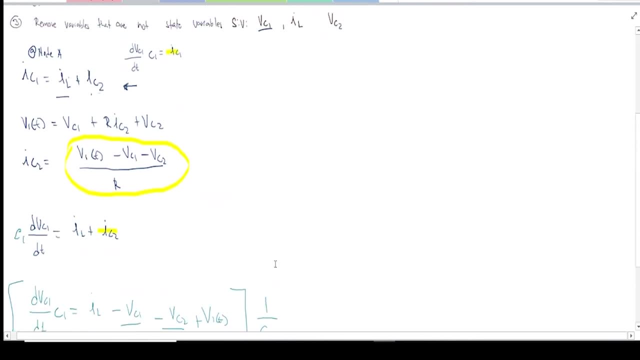 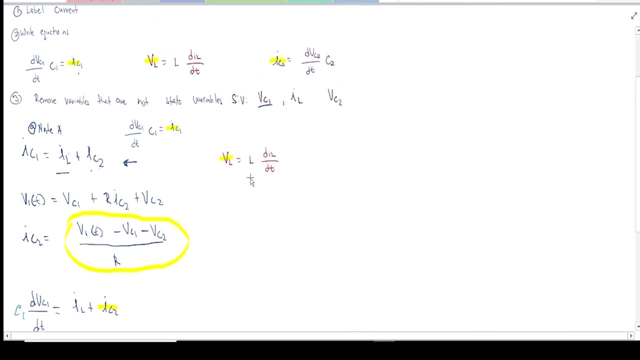 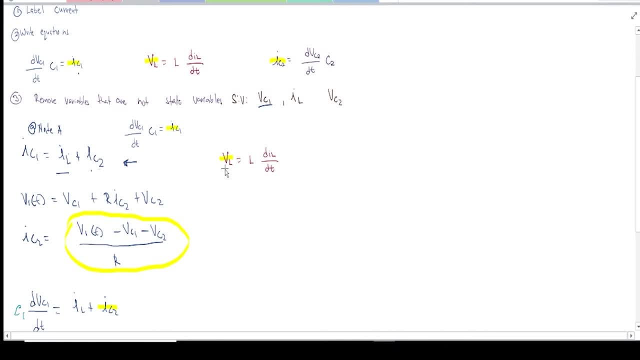 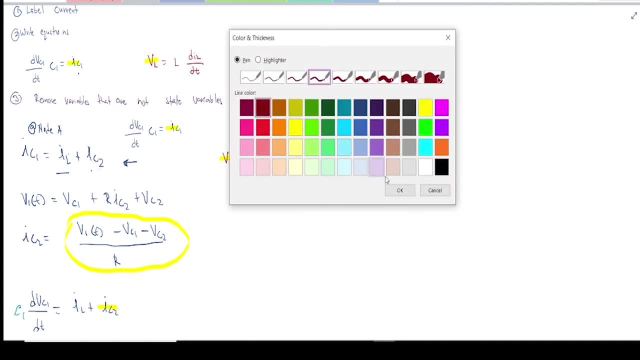 variable. okay, so we're working on this variable. okay, so we're working on this one in order to make it more organized. one in order to make it more organized. one in order to make it more organized and more easier for you to follow I'm and more easier for you to follow I'm. 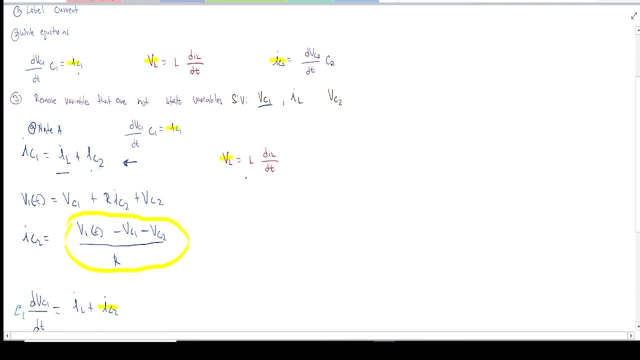 and more easier for you to follow. I'm going to use the same ink which is kind. going to use the same ink which is kind. going to use the same ink which is kind of rubbish. so let's begin analyzing of rubbish. so let's begin analyzing of rubbish. so let's begin analyzing this one. 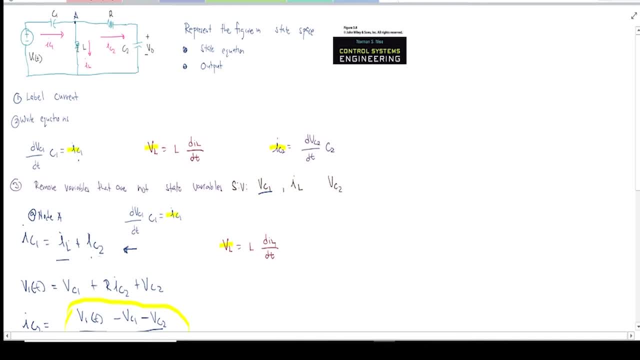 this one, this one. so our problem here is the voltage drop. so our problem here is the voltage drop. so our problem here is the voltage drop. we have to represent this in terms of. we have to represent this in terms of. we have to represent this in terms of state variables. again, let's think of: 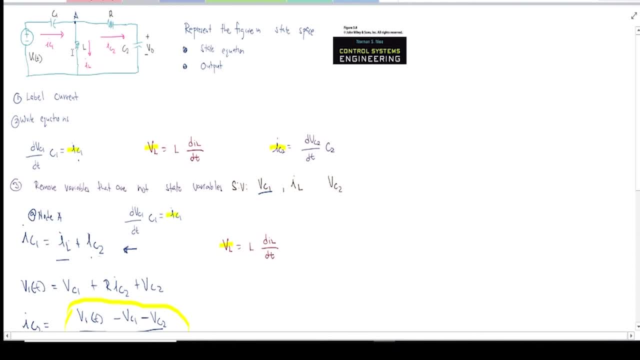 state variables again. let's think of state variables again. let's think of something that will make this BL into something, that will make this BL into something that will make this BL into state variable. let's imagine that we're state variable. let's imagine that we're. 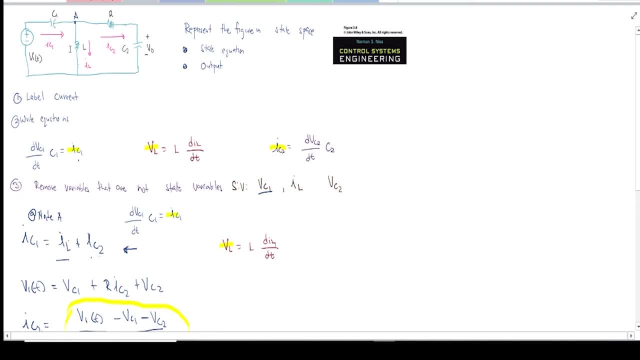 state variable. let's imagine that we're going to have a loop on this one in the going to have a loop on this one in the going to have a loop on this one in the first one. we're going to have a loop first one. we're going to have a loop on this one in the first one. it is easy if. 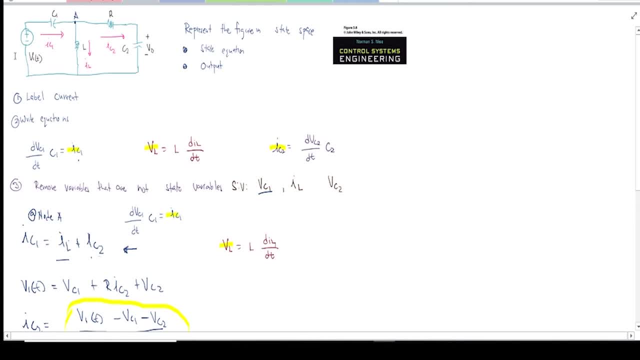 on this one it is easy. if on this one it is easy, if you have a loop on this one, because you, you have a loop on this one, because you, you have a loop on this one, because you have the input okay and then the voltage, have the input okay and then the voltage. 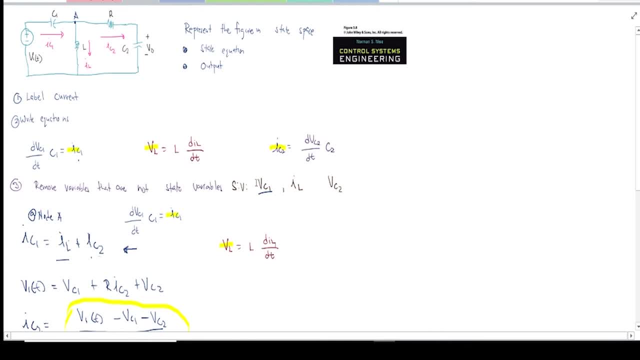 have the input, okay, and then the voltage drop would be BC1, which is a state drop, would be BC1, which is a state drop, would be BC1, which is a state variable, and then BL- you know, we're just variable. and then BL. you know, we're just. 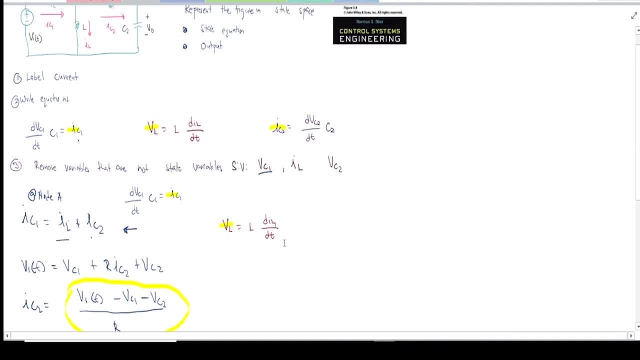 variable and then BL. you know, we're just going to isolate this, okay, so that we going to isolate this okay, so that we going to isolate this okay, so that we have the equation for the BL if we're have the equation for the BL if we're. 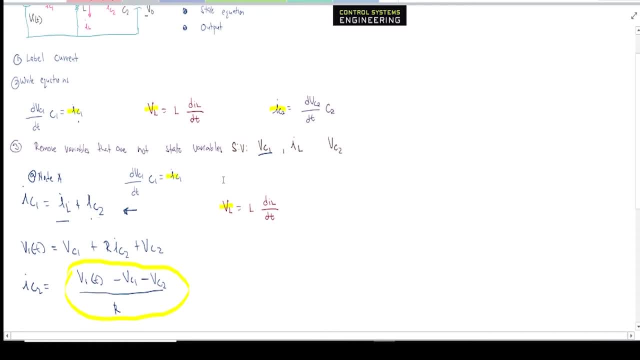 have the equation for the BL. if we're going to do that, look okay. so that's going to do that. look okay, so that's going to do that, look okay. so that's our equation for this one. just make sure, our equation for this one, just make sure. 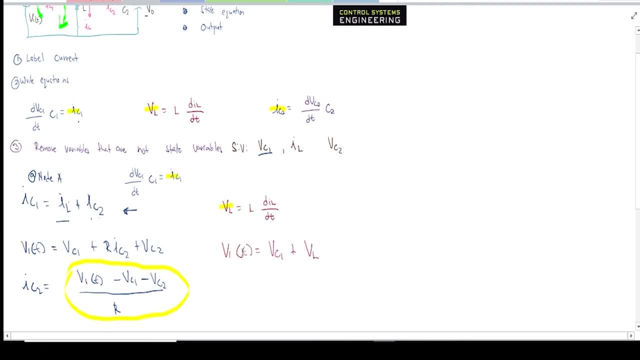 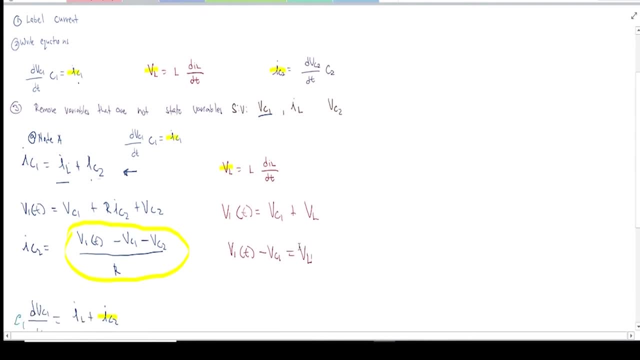 our equation for this one. just make sure that you have the correct equation also, that you have the correct equation also, that you have the correct equation also. again, be wary of your sign, okay. so now again. be wary of your sign, okay. so now again. be wary of your sign, okay. so now what we're going to do is just insert. 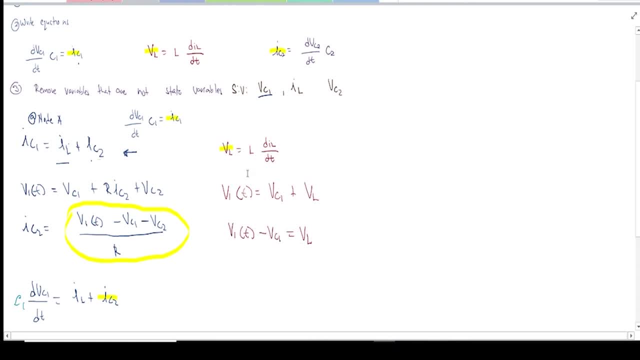 what we're going to do is just insert. what we're going to do is just insert this one, this one, this one, into into into this one, and then divide this by 1 over L- this one, and then divide this by 1 over L, this one, and then divide this by 1 over L, so that the other side of equation will. 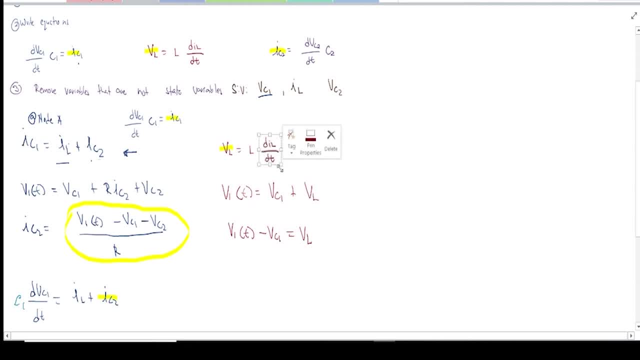 so that the other side of equation will, so that the other side of equation will be just this one, the one that I have in be just this one, the one that I have in be just this one, the one that I have in back, the same process that we did here. 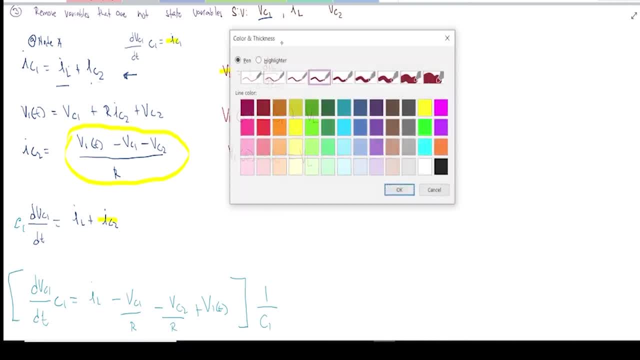 back the same process that we did here, back the same process that we did here. I'm just going to do it much more. I'm just going to do it much more. I'm just going to do it much more, faster again. what I'm going to do is I'm 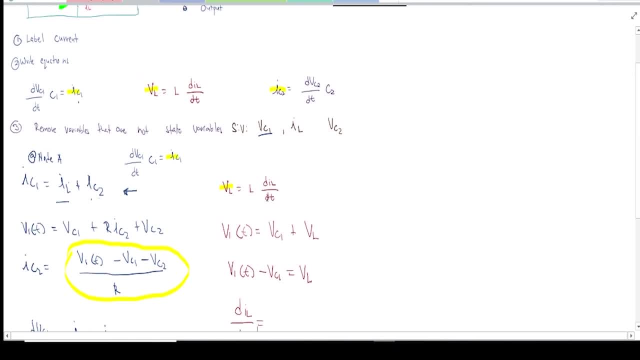 faster again. what I'm going to do is I'm faster again. what I'm going to do is I'm going to make it disorganized, starting going to make it disorganized, starting going to make it disorganized, starting from BC 1, I L, BC 2 and then in just 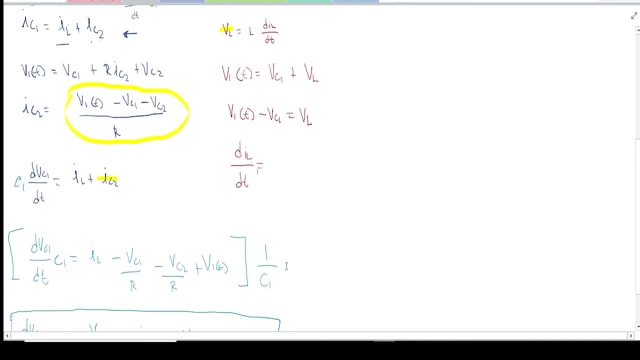 from BC 1 I L BC 2, and then in, just from BC 1 I L BC 2, and then in, just like what we did here, because this is like what we did here, because this is like what we did here, because this is critical or important in order for us to 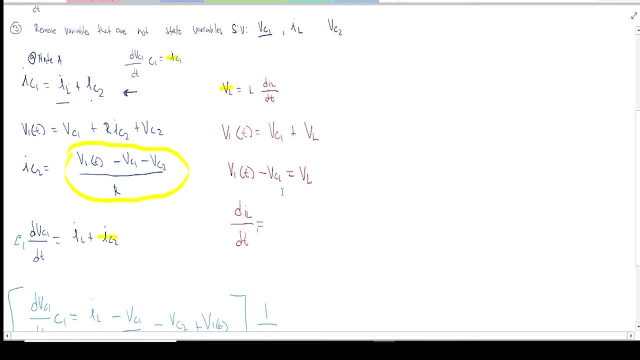 critical or important in order for us to critical or important in order for us to have the state equation because it is in. have the state equation because it is in. have the state equation because it is in the matrix form. okay, now we're done with the matrix form. okay, now we're done with. 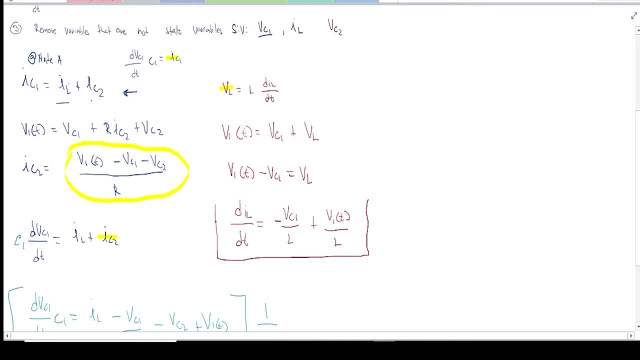 the matrix form. okay, now we're done with our second equation. so, as you can see our second equation, so as you can see our second equation. so, as you can see, this is just an easy step, but we only. this is just an easy step, but we only. 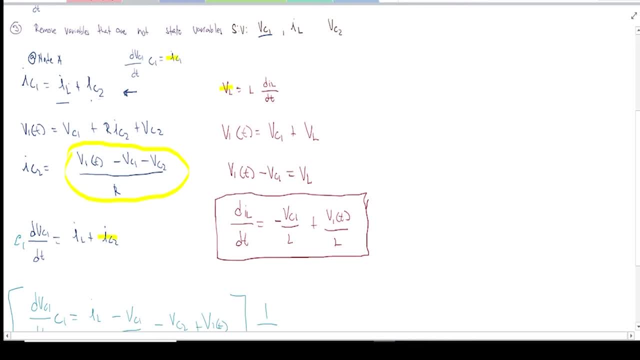 this is just an easy step, but we only think that we should be aware of. is that think that we should be aware of? is that think that we should be aware of? is that expressing the not state variable into a, expressing the not state variable into a. expressing the not state variable into a state variable. okay, the same pattern. 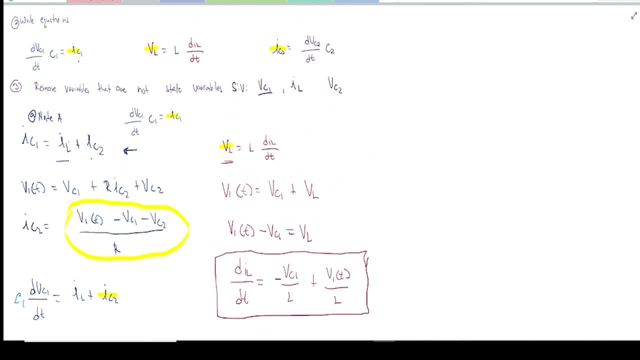 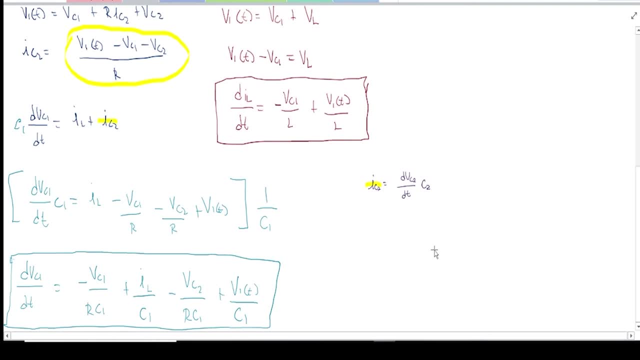 state variable: okay, the same pattern. state variable: okay, the same pattern. that with what we're going to use. okay, that with what we're going to use. okay, that with what we're going to use. okay, for our final equation, as you can see, for our final equation, as you can see. 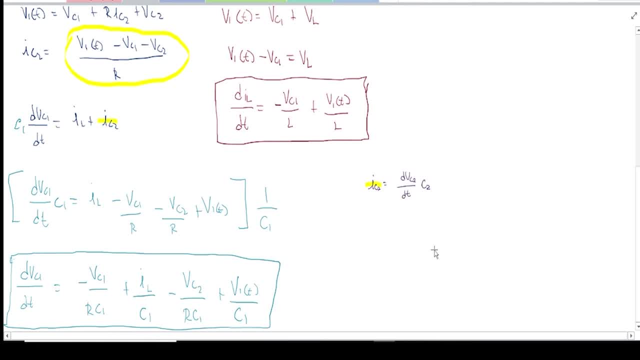 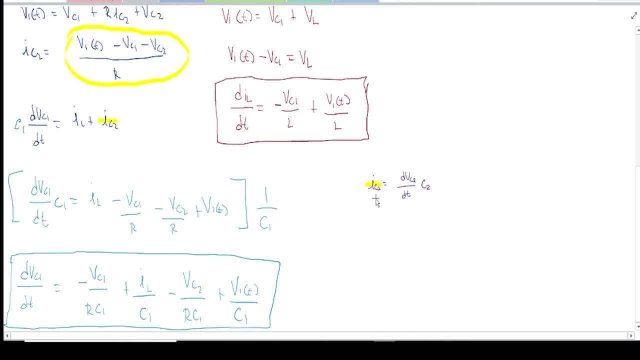 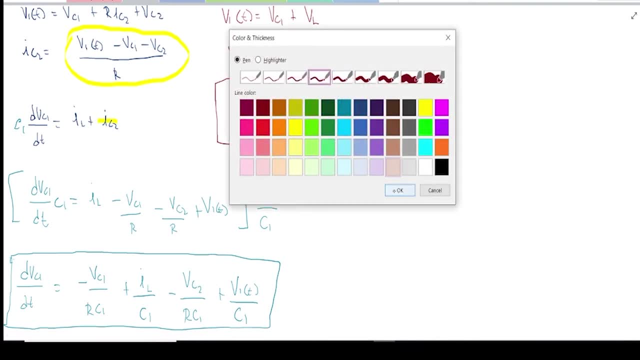 um next pattern would be again. um next pattern would be again: represent this current in the capacitor, represent this current in the capacitor, represent this current in the capacitor into a state variable, into a state variable, into a state variable. and again we already have state variable and again we already have state variable. 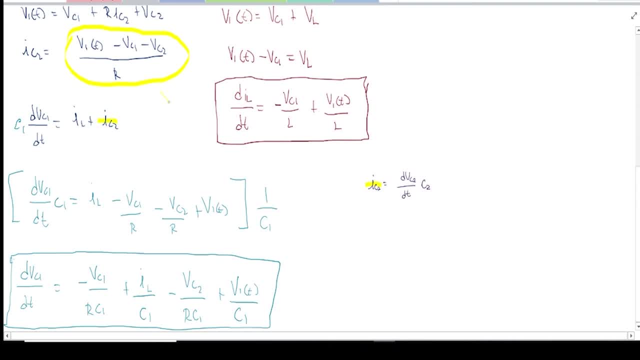 and again, we already have state variable for this one, for this one, for this one which is again, which is again, which is again. that's one, that's one, that's one, okay, okay, okay. so that's why it is critical that we, so that's why it is critical that we. 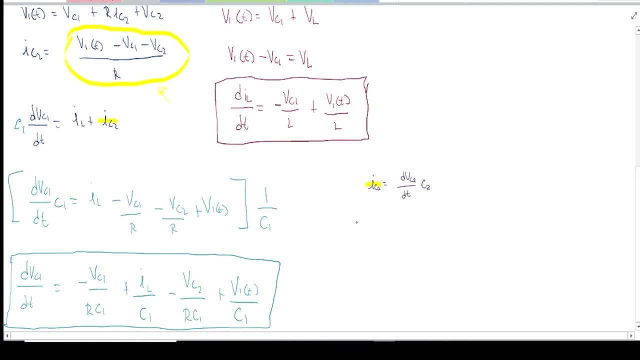 so that's why it is critical that we have the correct setup of equation, have the correct setup of equation, have the correct setup of equation. okay, okay, okay, what i'm going to do, what i'm going to do, what i'm going to do, is that i'm going to replace this. 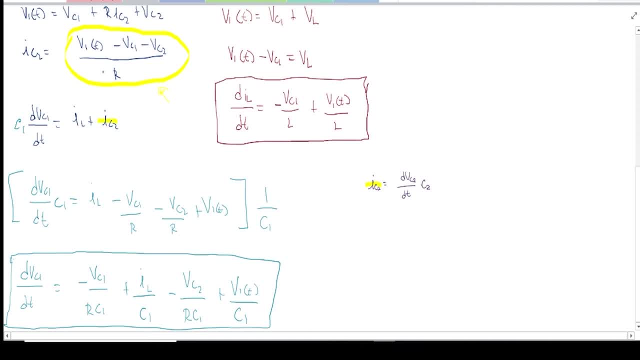 is that i'm going to replace this, is that i'm going to replace this ic2 by this one ic2 by this one ic2 by this one. okay, okay, okay, and then, and then, and then. i'm going to organize this starting from. i'm going to organize this starting from. 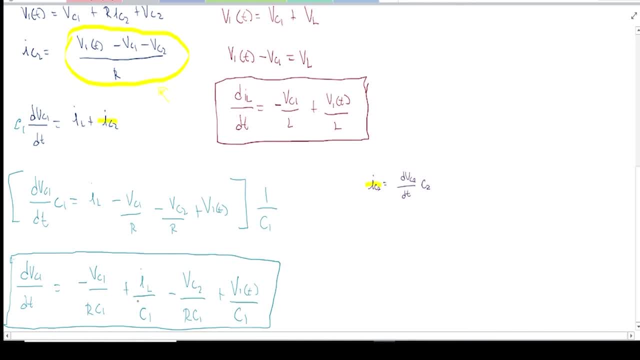 i'm going to organize this starting from vc1, vc1, vc1, il, il il, and then vc2, and then vc2, and then vc2, okay, and then i'm going to divide this. okay, and then i'm going to divide this. okay, and then i'm going to divide this by one over c2. 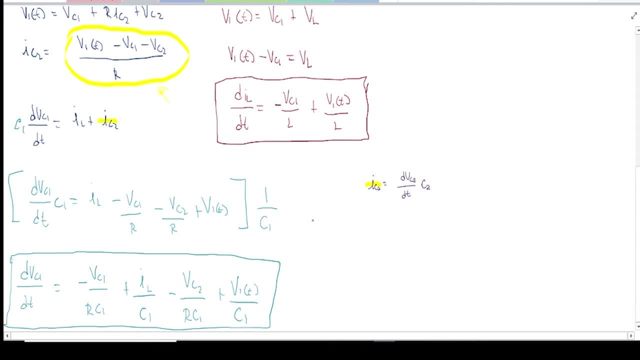 by one over c2, by one over c2- again same pattern by what we did here. again same pattern by what we did here. again same pattern by what we did here. our equation would now be: now we have the third equation, we have the third equation, we have the third equation. at this point we need to be silent. 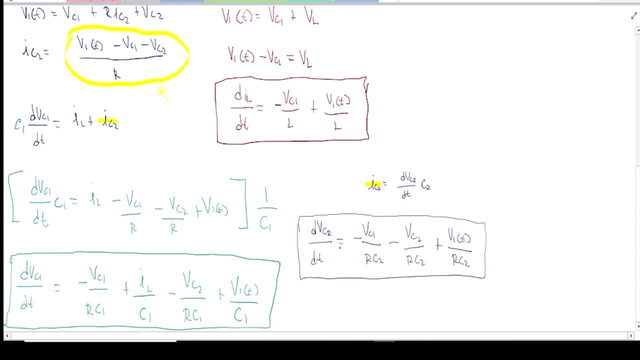 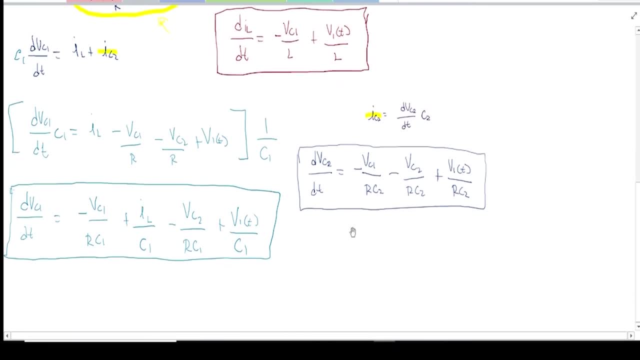 at this point we need to be silent. at this point, we need to be silent because, because, because you will hear a drum roll, you will hear a drum roll. you will hear a drum roll, because we're nearly done, because we're nearly done, because we're nearly done and we're just going to input this. 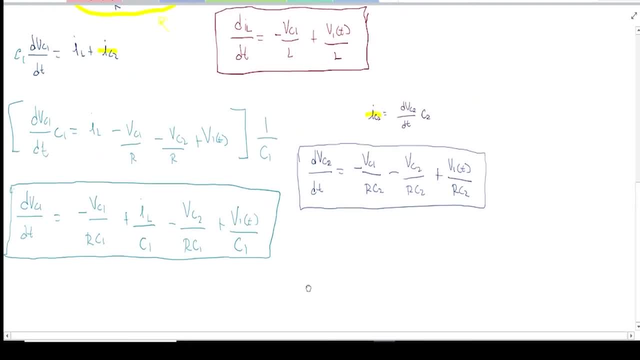 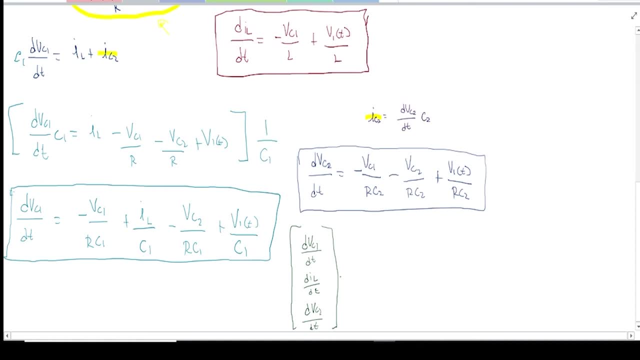 and we're just going to input this, and we're just going to input this in in in a matrix form. don't be so intimidated if you don't be so intimidated, if you don't be so intimidated if you encounter, encounter, encounter this one, this kind of one, because, um, at 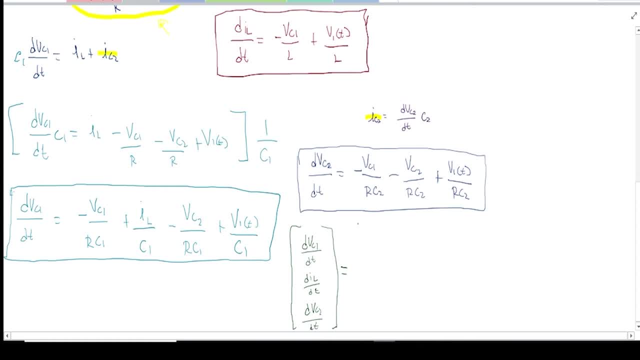 this one, this kind of one, because, um, at this one, this kind of one, because um, at first, first, first you will really feel intimidated, but as you will really feel intimidated, but as you will really feel intimidated, but as you go along, and then you go along, and then 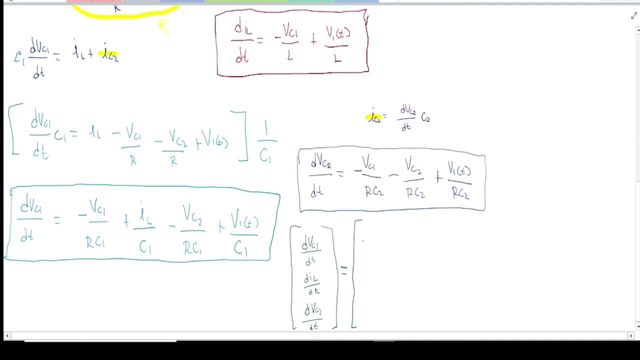 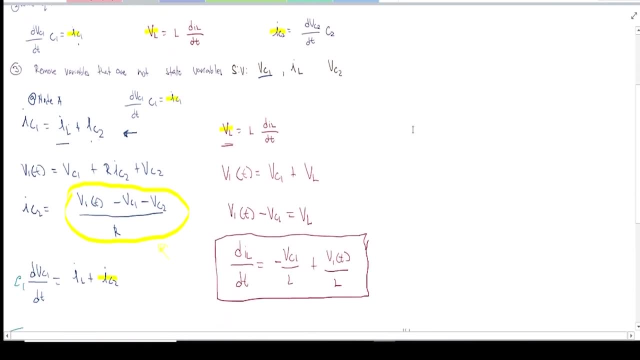 you go along and then practice. this is just easy practice. this is just easy practice. this is just easy. and also what's good about um and also what's good about um and also what's good about um. this book is that. this book is that. this book is that he has, or he has, techniques for making. 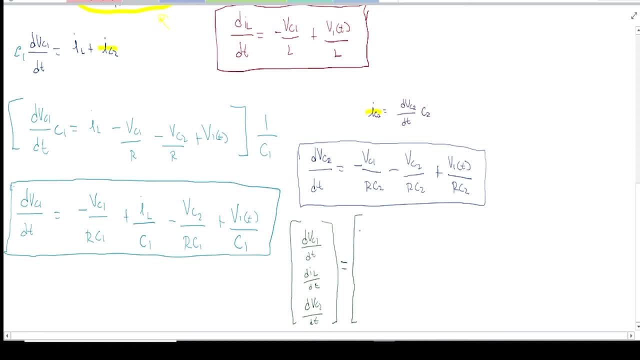 he has or he has techniques for making, he has or he has techniques for making it much more simplified. so, okay, let's make it in yellow this one. okay, let's make it in yellow this one. okay, let's make it in yellow this one would be for vc1. 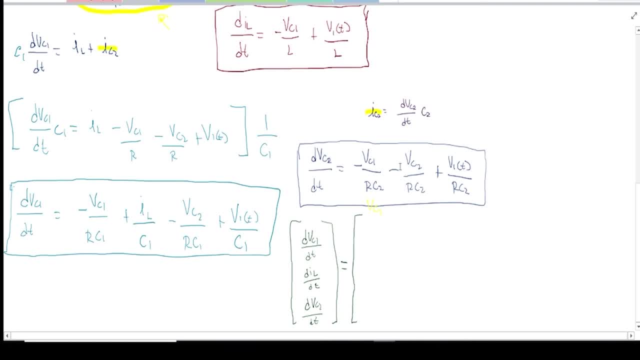 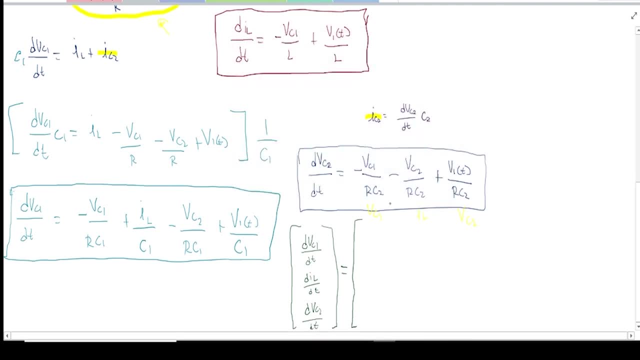 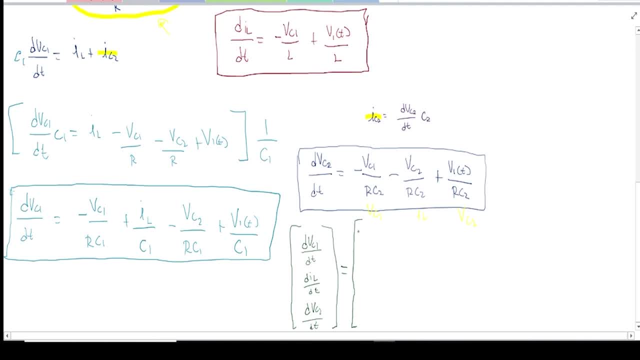 the vc1 would be. the vc1 would be: that's one, the first equation. that's one. the first equation, that's one. the first equation minus one minus one. minus one. rc1, rc1, rc1. next would be this one minus one over l. next would be this: one minus one over l. 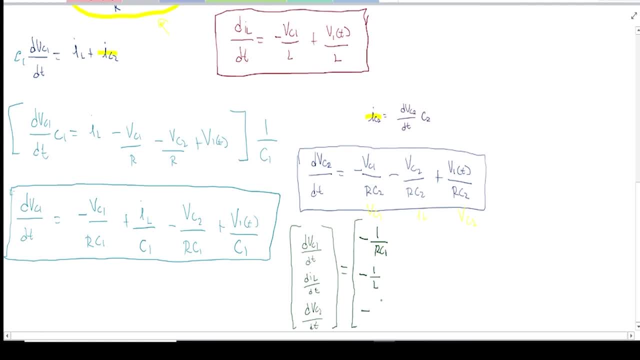 next would be this one minus one over l, and then the last one would be this one, and then the last one would be this one, and then the last one would be this one minus one over l. that's why putting it in the. and then the last one would be this one minus one over l. that's why putting it in the. 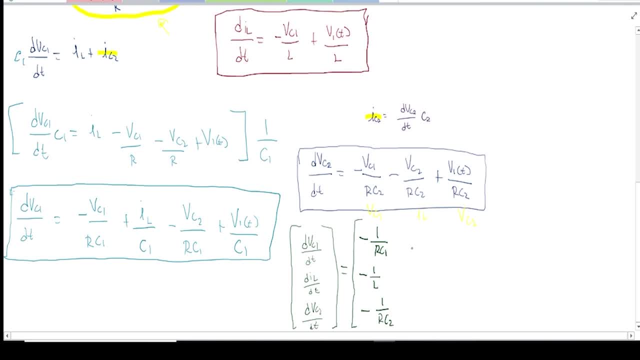 and then the last one would be this: one minus one over l. that's why putting it in the matrix form is just an easy steps. matrix form is just an easy steps. matrix form is just an easy steps. okay, now for il okay. okay, now for il okay. 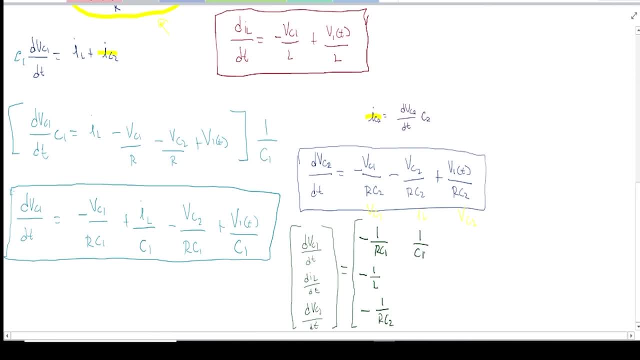 okay, now for il. okay, one over c1, one over c1, one over c1. there is no il here, so zero, same with. there is no il here, so zero, same with. there is no il here, so zero, same with this one, this one, this one i'm going to speed up the process with. 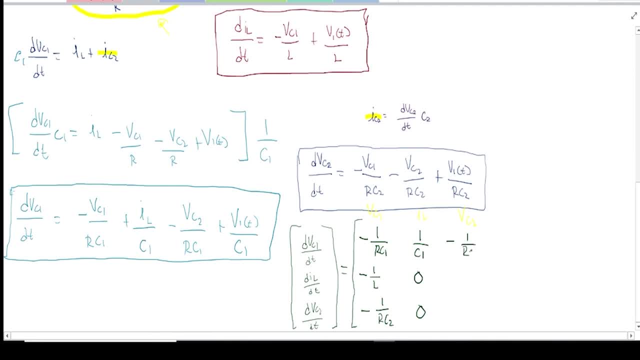 i'm going to speed up the process with: i'm going to speed up the process with the vc2: just look for their coefficient. the vc2- just look for their coefficient. the vc2: just look for their coefficient. okay, okay, okay. the next thing that we're going to do: 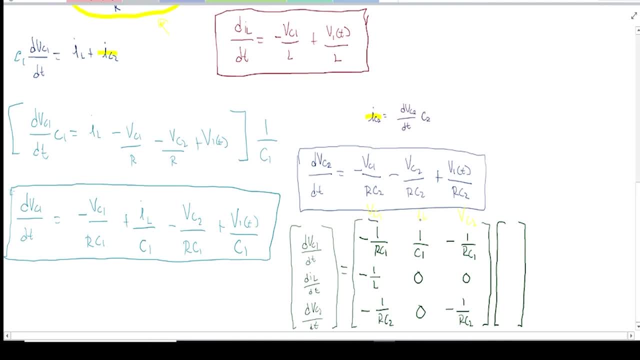 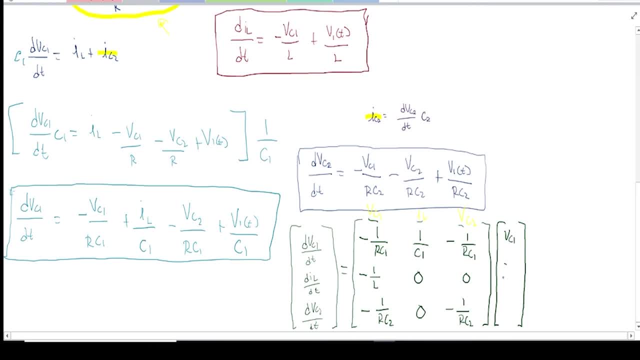 or the state variable we're just going to, or the state variable we're just going to put it here, put it here, put it here. so, starting from vc1, vc1, vc1, vc2, vc2, vc2, and maybe you're wondering how about this and maybe you're wondering how about this. 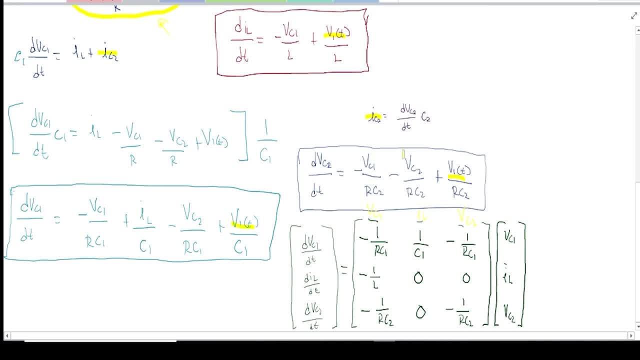 and maybe you're wondering: how about this one, one one, this one then this, this one then this, this one then this one, this one then this one? we're not just going to ignore this. we're not just going to ignore this. we're not just going to ignore this. instead, we're just going also to 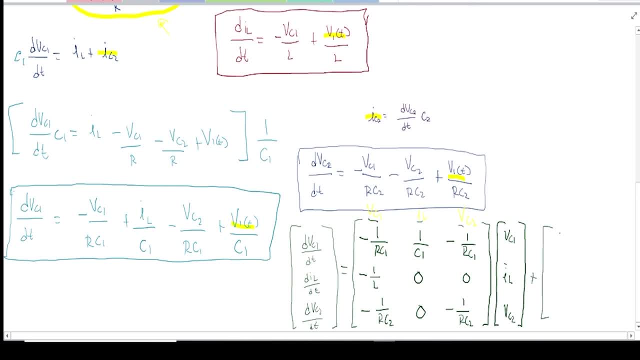 instead, we're just going also to, instead we're just going also to put it here, put it here, put it here: the same process, the same process, the same process for efficient, for efficient, for efficient, and then, since it is just alone, or v1d, and then, since it is just alone, or v1d. 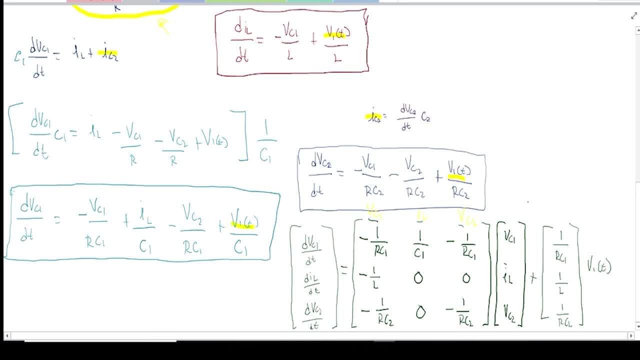 and then, since it is just alone or v1d, we're just going to um, we're just going to um, we're just going to um, put it here okay, put it here okay, put it here okay. so again, so again, so again, um, as i said, 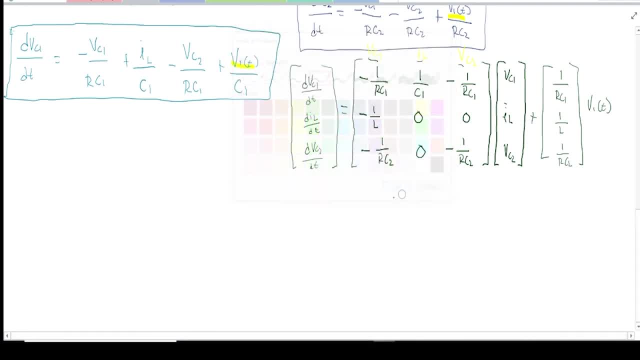 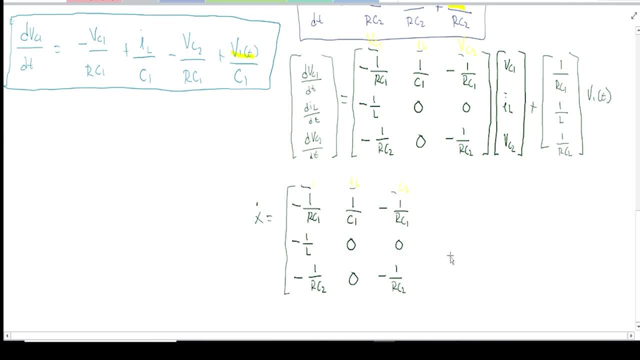 this one, this one i'm just going to copy: and then x the meaning of this one is, and then x the meaning of this one is. and then x the meaning of this one is that um, that um, that um. variable x with respect to time: see so. 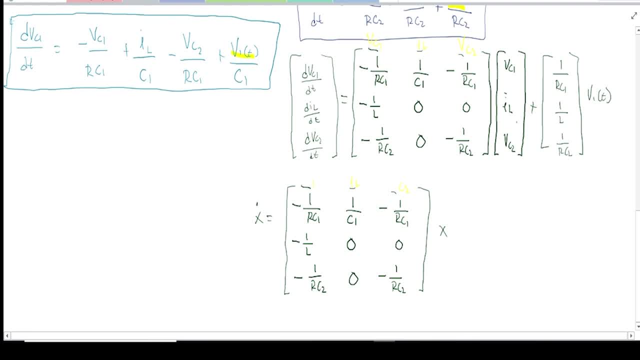 variable x with respect to time: see so variable x with respect to time: see so the variable x would be this one. the variable x would be this one. the variable x would be this one. imagine that they will have just dpdp. imagine that they will have just dpdp. 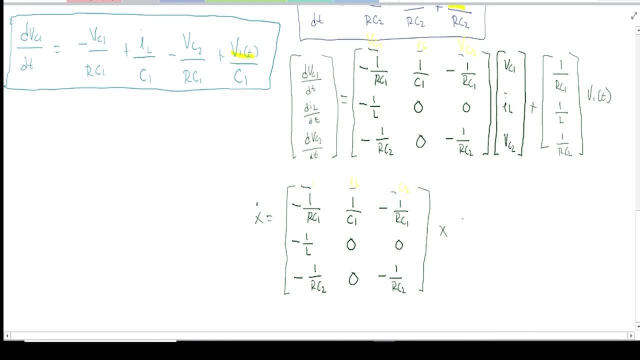 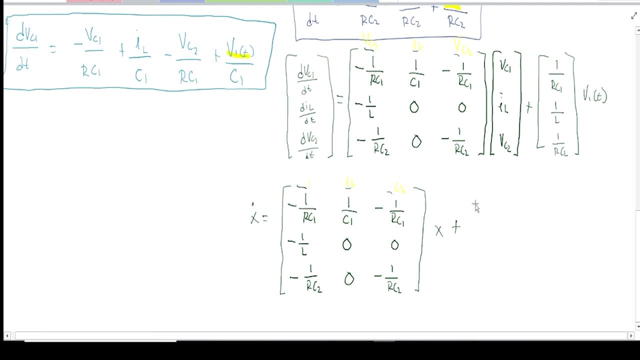 imagine that they will have just dpdp- okay, and then x would be against this, okay, and then x would be against this, okay, and then x would be against this, one, one one. so, as you can see, um, it's just easy. so, as you can see, um, it's just easy. 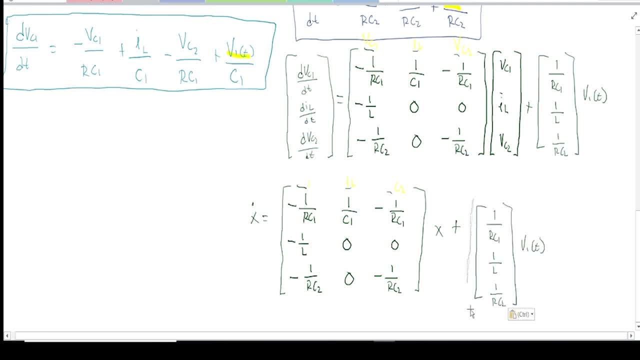 so, as you can see, um, it's just easy and it's also inspiring that, and it's also inspiring that and it's also inspiring that. you know, this kind of concept is very. you know, this kind of concept is very. you know, this kind of concept is very important and also very dangerous. 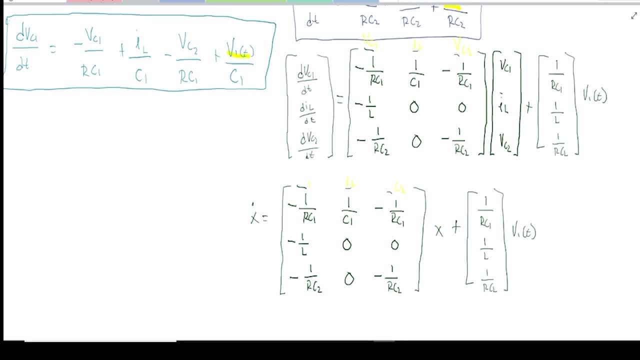 important and also very dangerous. important and also very dangerous because you know this kind of concept, because you know this kind of concept, because you know this kind of concept is used in launching missiles and for our is used in launching missiles and for our is used in launching missiles and for our last step would be: 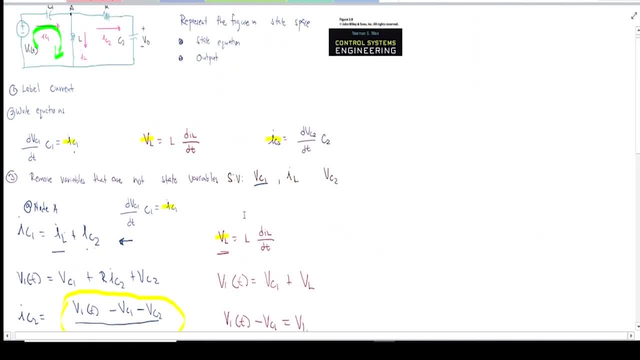 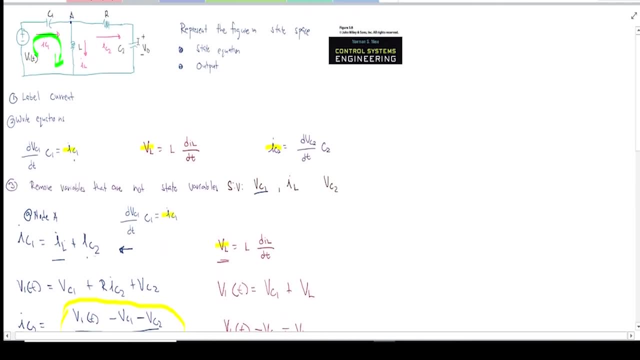 last step would be. last step would be: um output, um output, um output of this one, of this one, of this one. so the output for this one is so the output for this one is. so the output for this one is vc2, vc2, vc2, which is again a state variable. 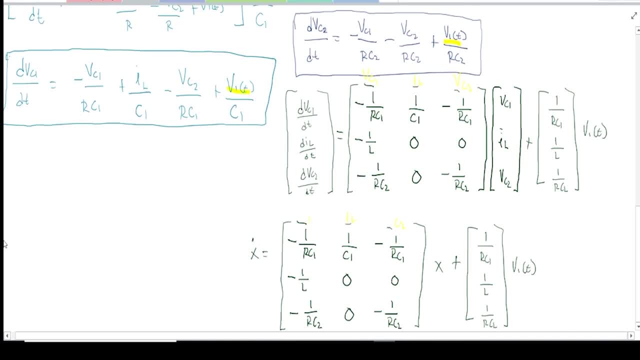 which is again a state variable, which is again a state variable. so we do that here, we do that here, we do that here: vc2, vc2, vc2: it equals to vo, it equals to vo, it equals to vo. okay, so, therefore, okay, so, therefore okay, so therefore vo. 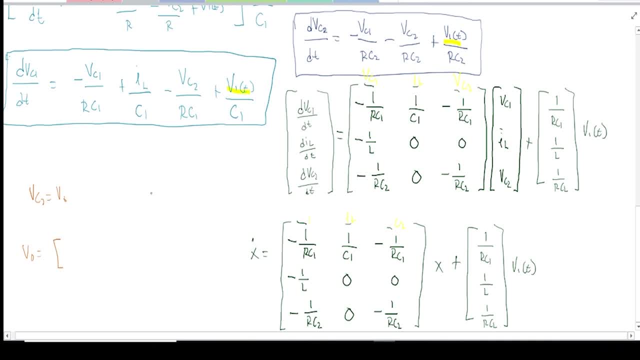 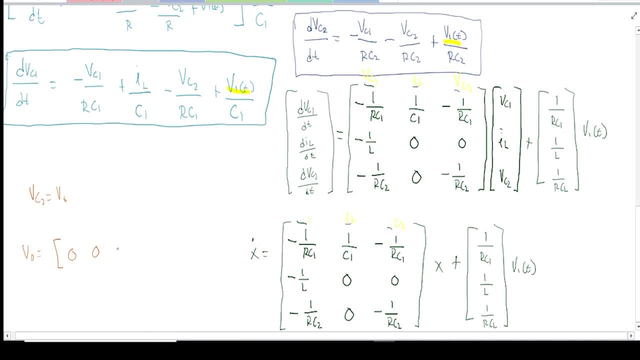 there is no current in the inductor. so there is no current in the inductor. so, which was zero? which was zero, which was zero. however, there is vc2, which has a. however, there is vc2, which has a. however, there is vc2 which has a coefficient of one. 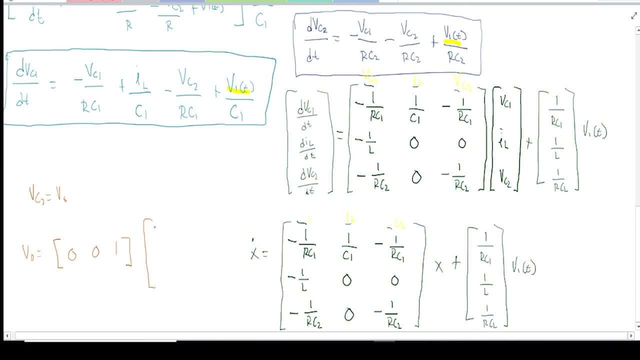 coefficient of one, coefficient of one. okay, okay, okay, and then you have to, and then you have to, and then you have to accept. okay, so that's it okay, so that's it. so in this video, you learn how to. so in this video, you learn how to. 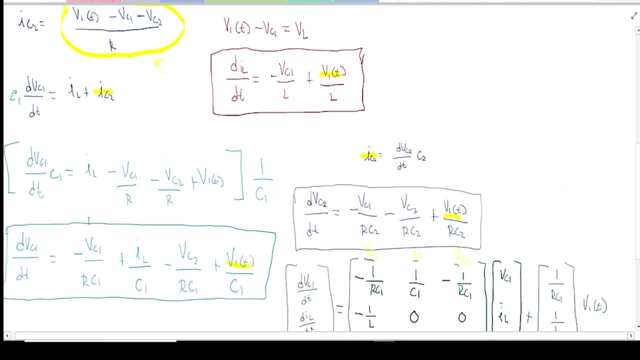 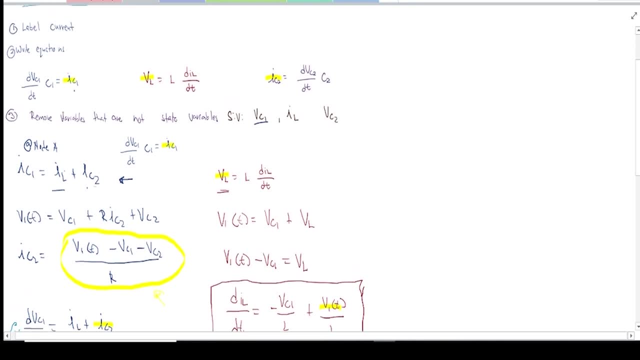 so in this video you learn how to make state equation and then the output make state equation, and then the output make state equation, and then the output: um, um, um. the this one, just remember that. the this one, just remember that. the this one just remember that the goal of this one is just to remove. 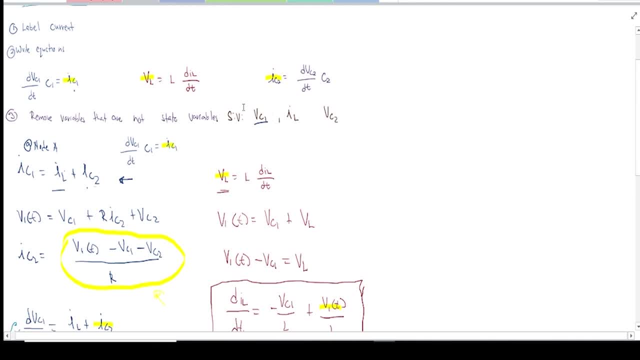 the goal of this one is just to remove. the goal of this one is just to remove the variables that are not state, the variables that are not state, the variables that are not state variables, variables, variables, and then and then, and then change it with the state variables. 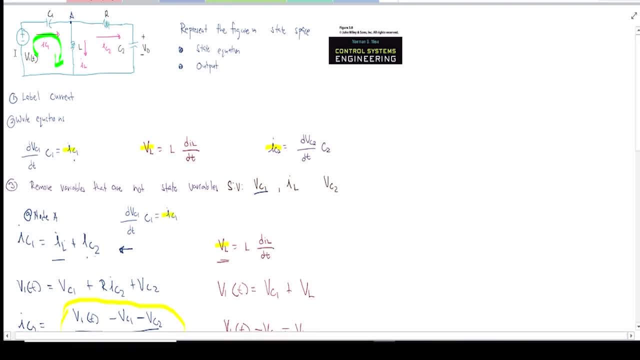 change it with the state variables, change it with the state variables. so again, so, again, so again. in this video you learn how to solve. in this video, you learn how to solve. in this video you learn how to solve this, this, this. so if you learned, please hit the like. 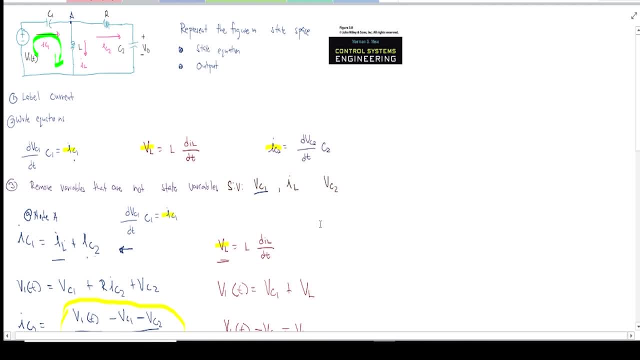 so, if you learned, please hit the like. so, if you learned, please hit the like button, button, button, subscribe and then subscribe, and then subscribe and then thank you for watching. caveat. be careful of this topic. caveat, be careful of this topic. caveat be careful of this topic because 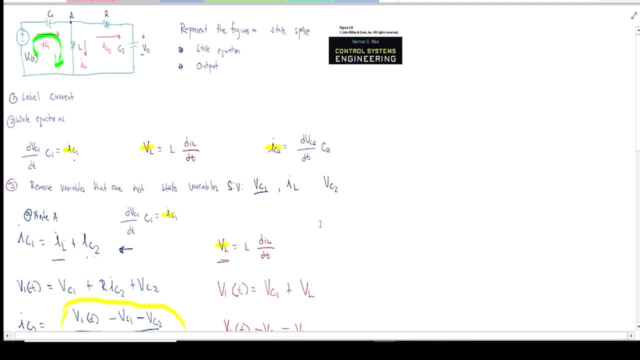 because, because you might know this topic, you might know this topic. you might know this topic as an equation used for missiles, as an equation used for missiles, as an equation used for missiles. okay, okay, okay, bye, bye.